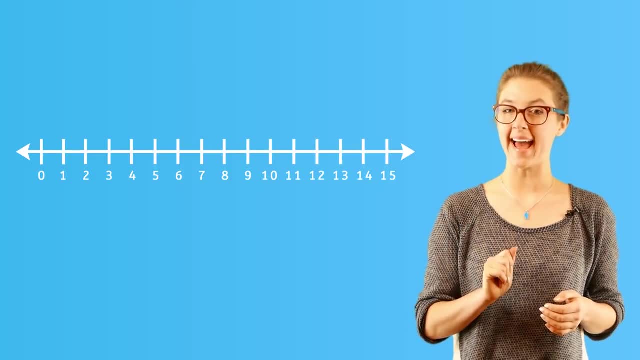 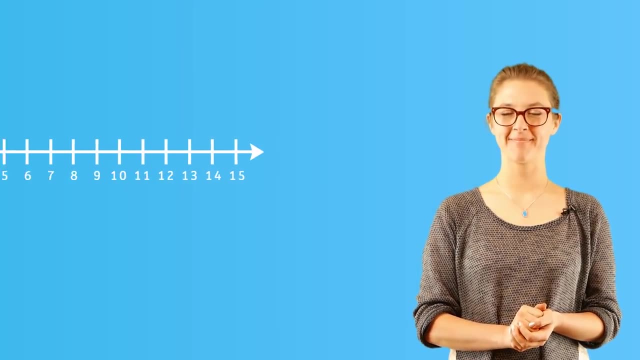 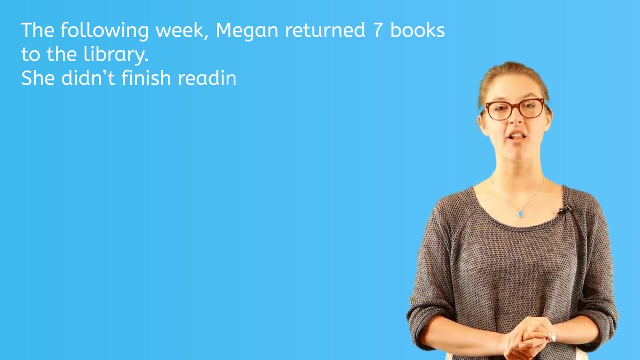 Yes, you got it, Since we moved right when we added we will move left to subtract. Here's a word problem to prove it. The following week Megan returned seven books to the library. She did not finish reading all of them. 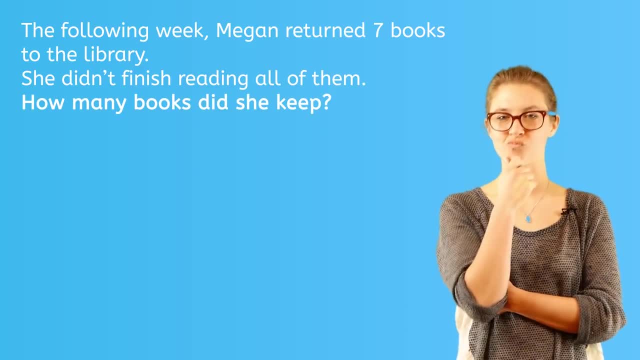 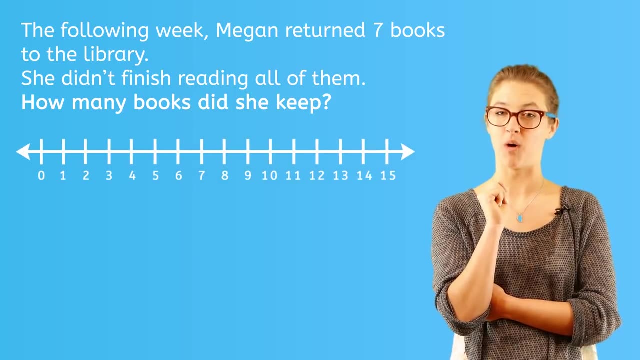 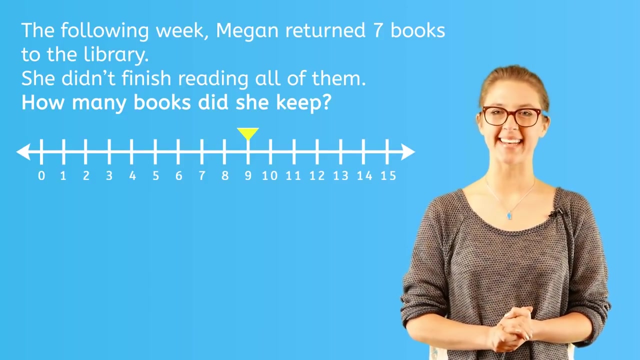 How many books did she keep? Hmm, Well, we know from the other problem that Megan borrowed a total of nine books, So we'll start at nine. on the number line, She returned seven books, so that means Megan has less books after her visit to the library. 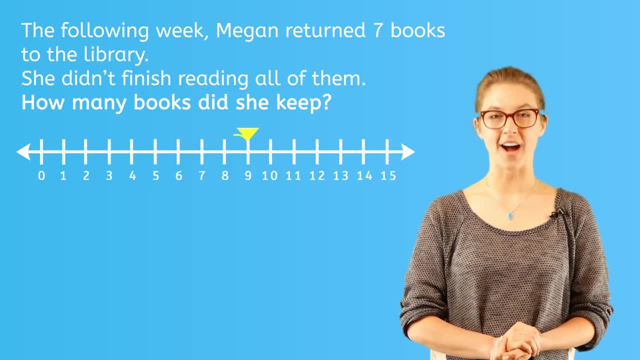 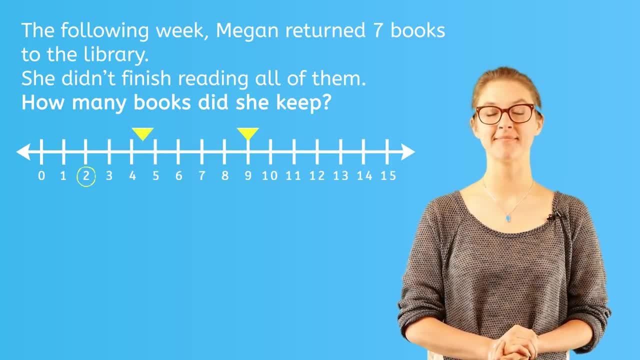 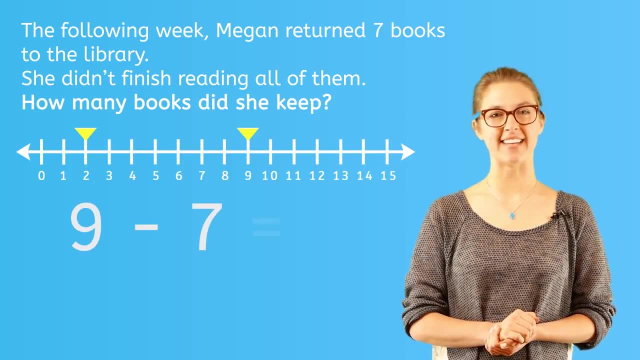 One, two, three, four, five, six. We'll subtract by moving left. One, two, three, four, five, six. We'll subtract by moving left Seven times. That leaves Megan with two books. That makes sense, since nine minus seven is two. 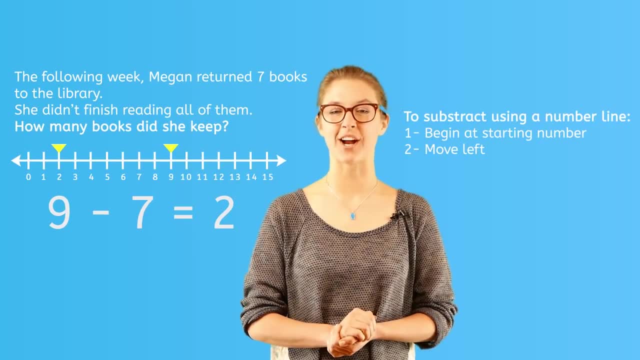 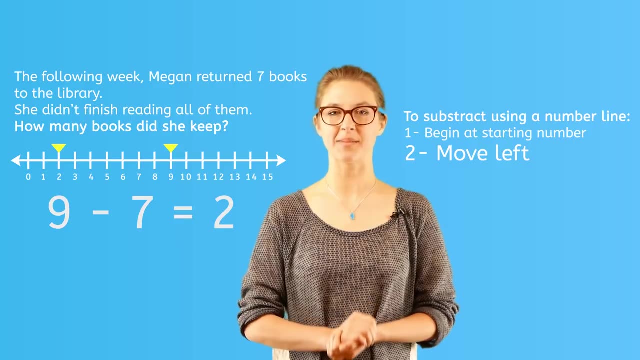 Just like adding. when we use a number line to subtract, we start at the number we were originally given and then we move left on the number line, however much we are subtracting by. After that is finished, we are at the end. 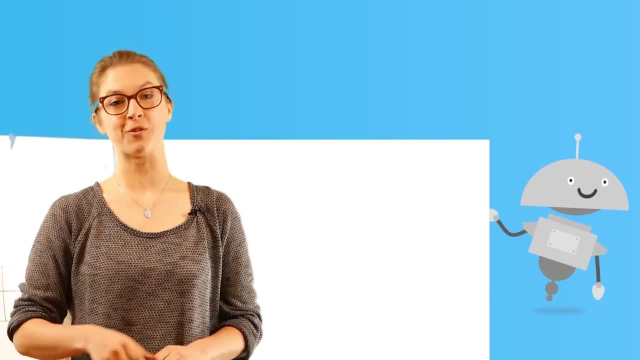 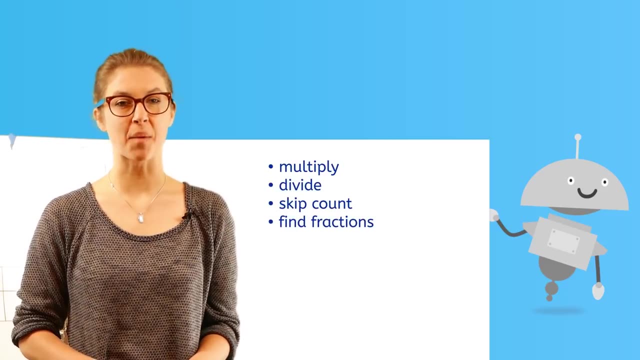 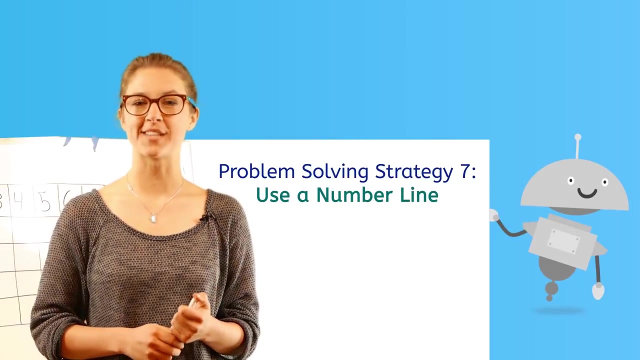 After that is finished, we are at the end. Number lines can also be used to solve problems where you'll need to multiply or divide, skip, count, find fractions, compare measurements and even to calculate differences in time. Solve the math word problems in our fun online games and quizzes. 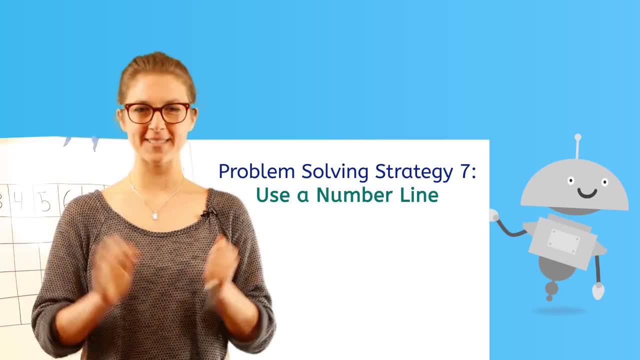 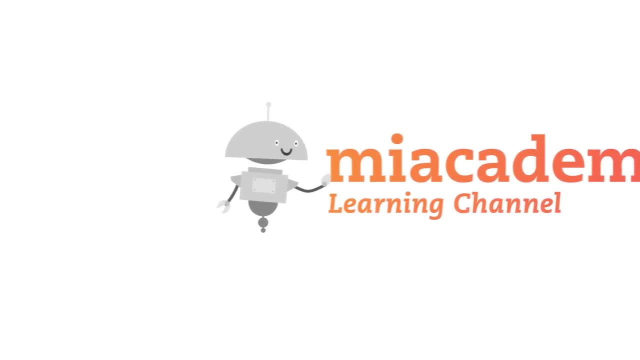 Keep practicing problem solving and remember to always be clever. If you had more than 15 words, pick one of the following methods. When you're done with your problem solving, you'll have to do the following three things. Then you'll need to use the word problem solving again. 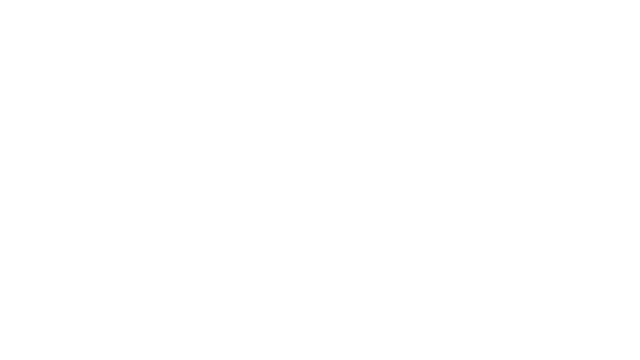 It's best to know your modeler because you will remember the problem you are solving At the end of the term. it's best to know the problem you're trying to solve. When you're done with your problem solving, you'll learn the problem you're trying to solve. 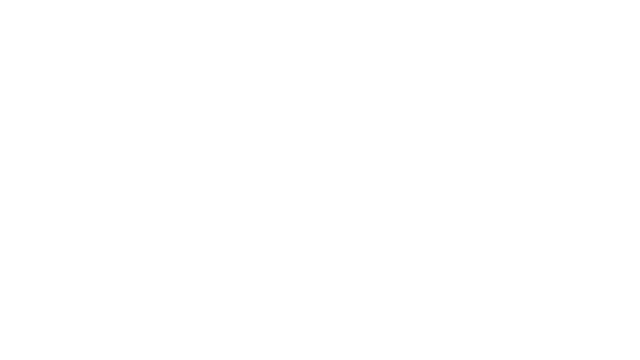 Then you'll need to apply the problem if it's something that you're not really sure you're doing, Remember that you can solve problems in every way. So this is the end of our lesson. Thank you for watching and if you liked this video. please give us a thumbs up. See you next time, bye, bye.